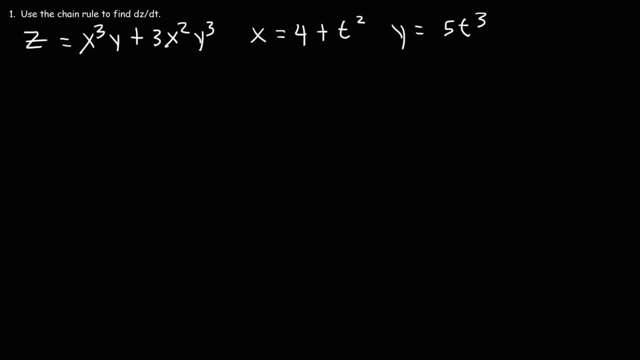 Let's work on this problem. Use the chain rule to find dz, dt. How can we do this? Well, we need to use partial derivatives. So z is a function of x and y, as we can see here, And x is a function of t. x is equal to 4 plus t, squared rather, And y is also a function of t. 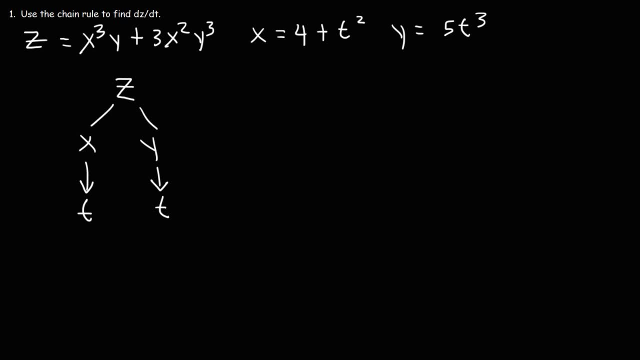 So to find dz- dt, first we need to find the partial derivative of z with respect to x. So basically we're going in this branch of the tree diagram And then we need to find dx- dt. Notice that we're not looking for the partial derivative of x with respect to t. 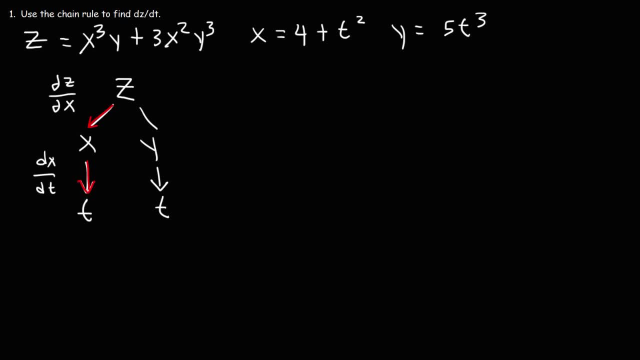 because x only has one variable, t. z has two variables, x and y. So we have to take the partial derivative of z, but not for x. Now we need to take this branch to get to t, So we need to find a partial derivative of z with respect to y. 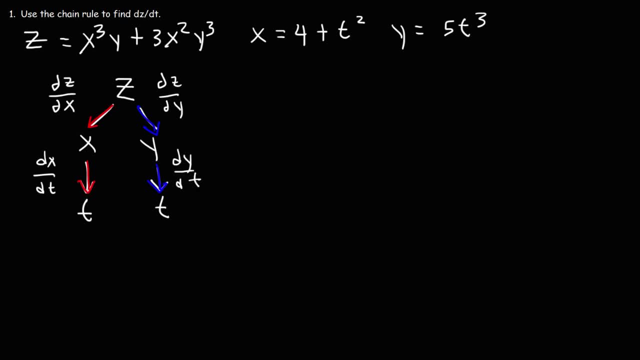 And then we need to find the partial derivative of z with respect to y, And then we need to find the partial derivative of z with respect to y, And then dy, dt. So now we can write the formula dz. dt is going to be the product of 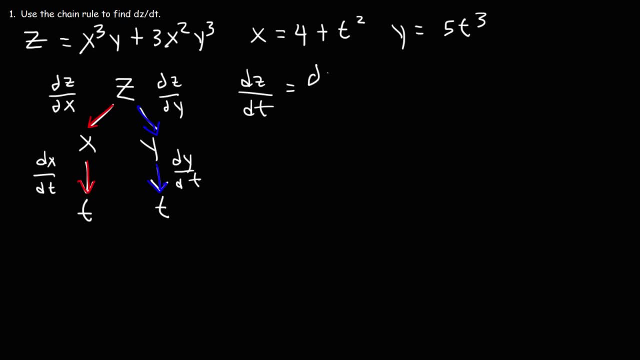 these two values. So that's the partial derivative of z with respect to x times dx dt, plus the partial derivative of z with respect to y. So we're going in this branch. And then times dy dt. So that's the formula we need to use in order to get dz dt. 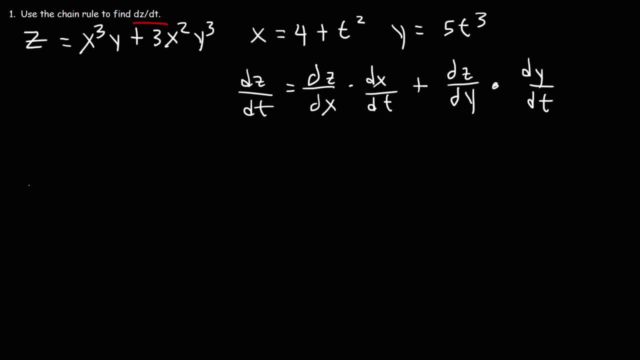 So let's start with this, So the partial derivative of z with respect to x. we can call that z sub x, if you want to. We're going to differentiate this function, but we're going to keep y as a. we're going to treat y as a constant. 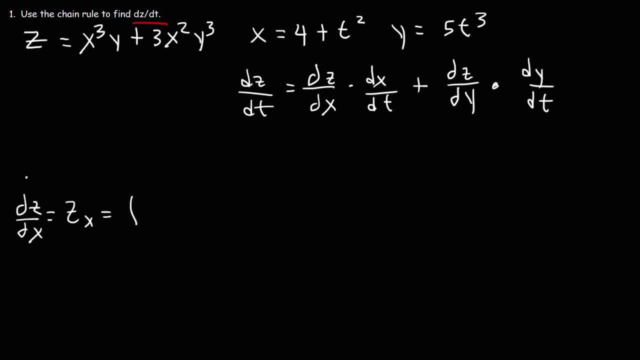 And differentiate only x. So the derivative of x cubed is 3x squared. y is a constant, so we're just going to rewrite it. The derivative of 3x squared, that's going to be 3 times 2x, So that's 6x And y cubed. we're going to treat that as a constant. 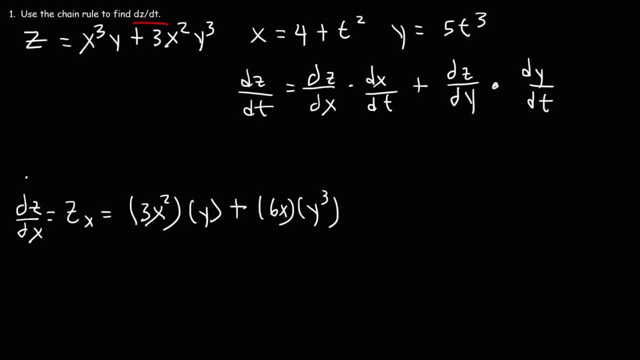 So we're just going to rewrite it. So now let's move on to the next one. Let's calculate the partial derivative of z with respect to x. So we're going to take the partial derivative of z with respect to y, So that's going to be z sub y. 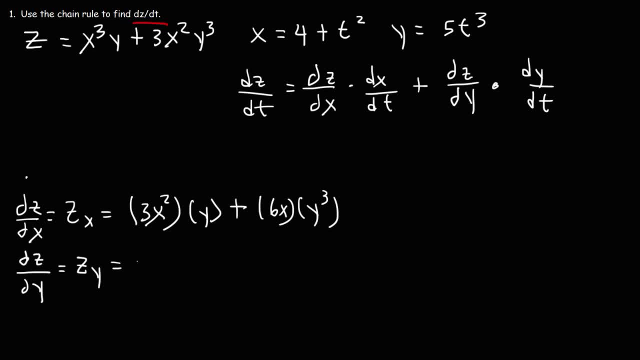 So we're going to treat x as a constant. So we're going to rewrite x cubed, And then we're going to take the derivative of y with respect to y. That's going to be 1.. Keep that as a constant, So that's going to be 3x squared. 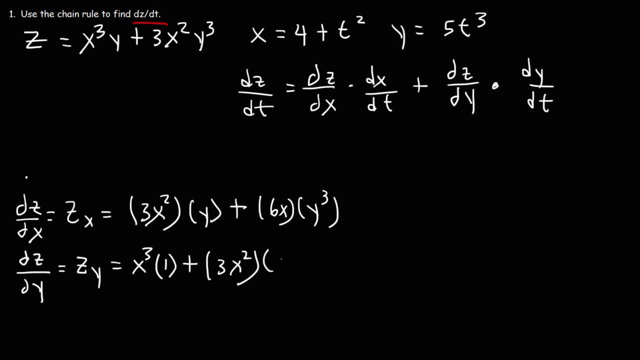 And then differentiate y cubed, So that's going to be 3y squared. So this simplifies to x cubed plus 9x squared, y squared. So now we need to determine dx, dt and dy dt. So x is 4 plus t squared. 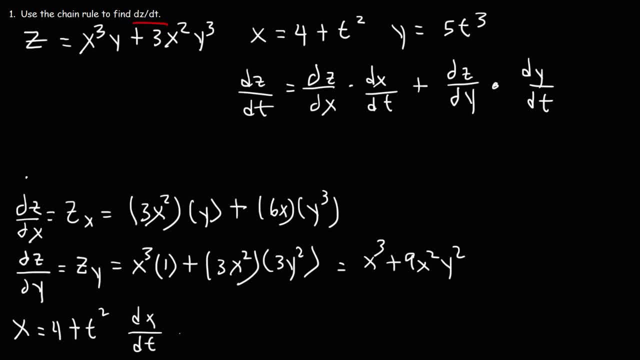 dx dt, the derivative of x with respect to t, it's going to be 2t. Now y is 5t cubed, So dy dt is going to be 5t, 5 times the derivative of t cubed, which is 3t squared. 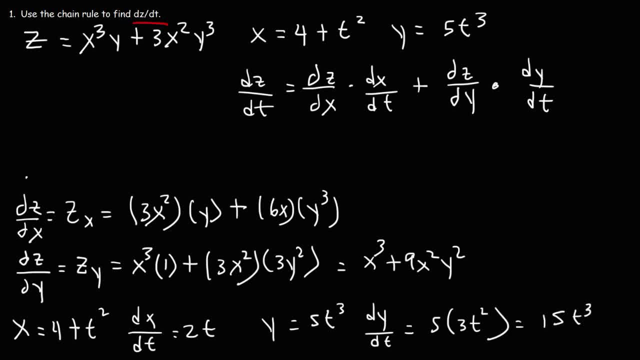 And so 5 times 3,, that's 15.. So now we have everything that we need. So let's plug it into this formula: dz, dt, that's going to be the partial derivative of z with respect to x. So that's everything that we see here. 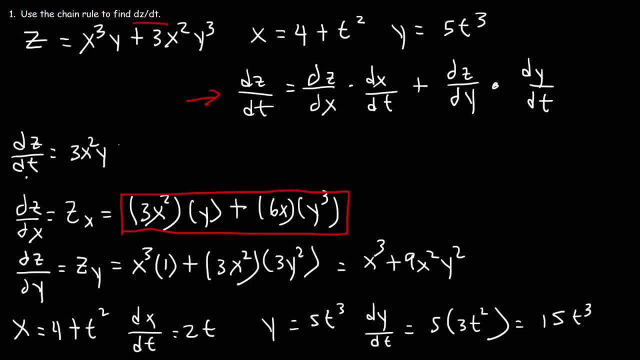 That's going to be 3x squared y plus 6x y cubed. Next, we're going to multiply that by dx, dt, which is here. it is 2t, So let's put this in brackets. 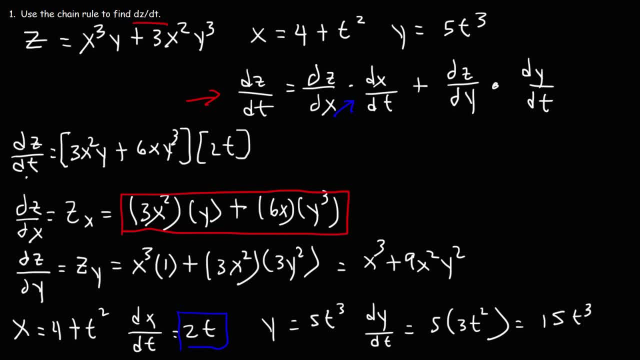 and then multiply this by 2t. Next we have the partial derivative of z with respect to y, and that is this answer here. So that's x cubed plus 9x squared, y squared, And then we have dy dt. 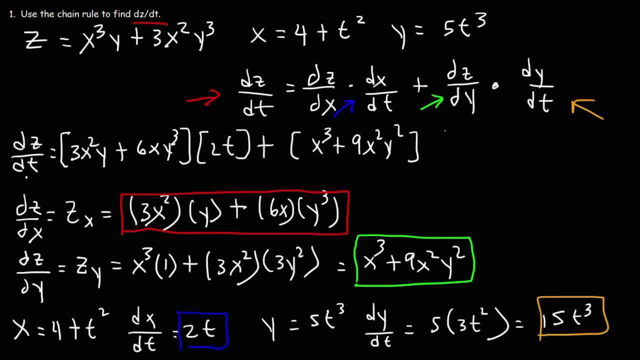 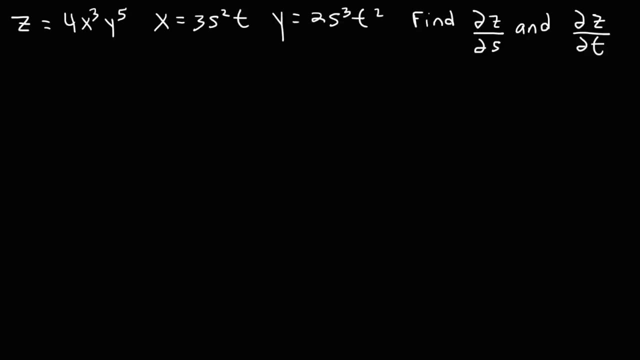 which is 15t cubed. So I'm going to leave the answer in this form. But this is it. This is dz, dt. So that's how we could use the chain rule to find it. Now let's move on to our next problem. 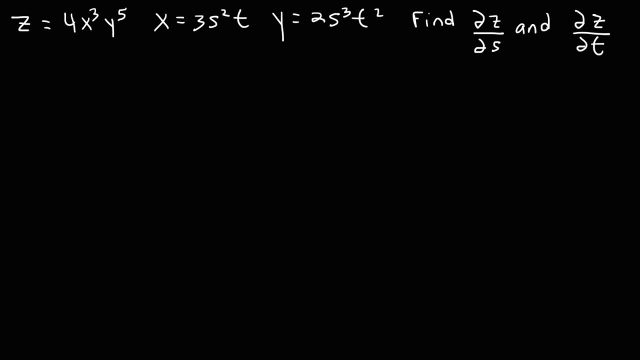 We're given the functions z, x and y and we're going to use the chain rule to find z, x and y And we need to find the partial derivative of z with respect to s and the partial derivative of z with respect to t. 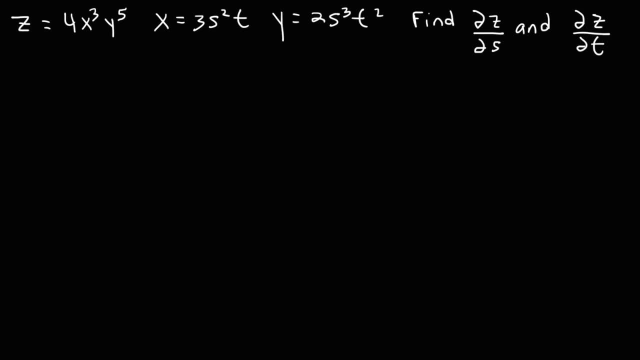 Now, this problem is similar to the last problem, but the only difference is that in the last problem, x was a function of t only, But this time x is a function of s and t, and y is a function of s and t as well. 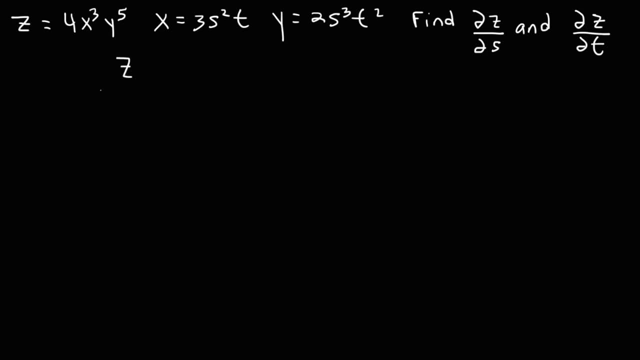 So we need a new tree diagram. So, starting with z, we see that z is a function of x and y, And x is a function of s and t, And the same is true for y. So let's start by finding this particular partial derivative. 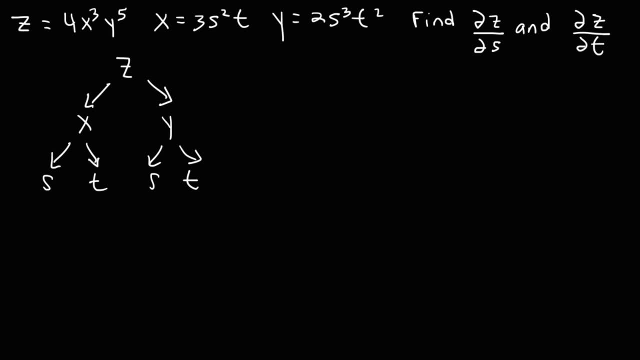 Let's write the formula for it. So we need to focus on everywhere we see an s, So we're going to follow these particular branches. So it's going to be the partial derivative of z with respect to x times the partial derivative of x with respect to s. 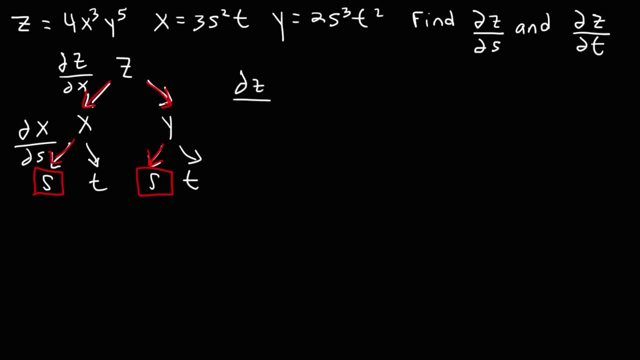 So let's write that. So the partial derivative of z with respect to s is going to be the partial derivative of z with respect to x times the partial derivative of x with respect to s. Now for the other side. So this is going to be the partial derivative of z with respect to y. 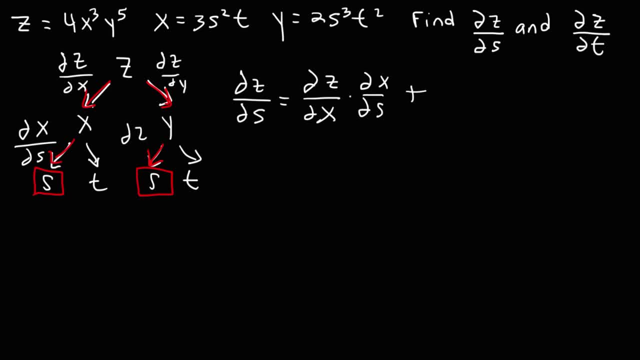 And then we have the partial derivative of y with respect to s. So let's write that in the formula here. So that's the equation that we need to use in order to get the partial derivative of z with respect to s. So let's begin. 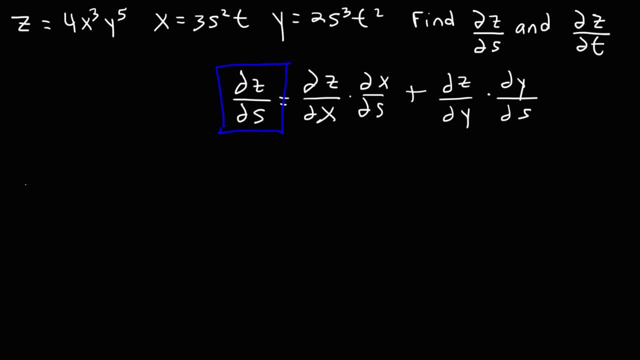 So let's start with this one, The partial derivative of z with respect to x. So we're going to treat y as a constant. We're going to differentiate the x part. The derivative of x cubed is 3x squared, So we have 4x squared. 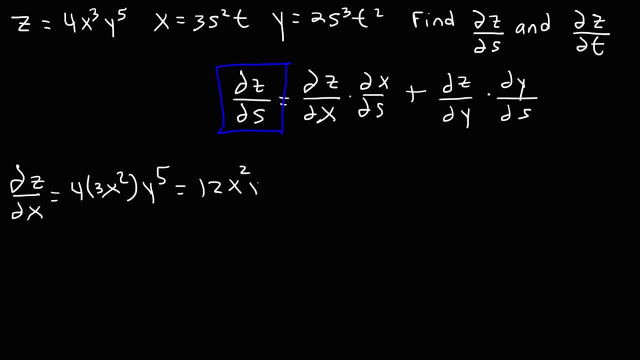 So 4 times 3,, this is going to be 12x squared y to the 5th power. Now let's find the next one, The derivative of x with respect to s. So we're using this, So t. we're going to treat that as a constant. 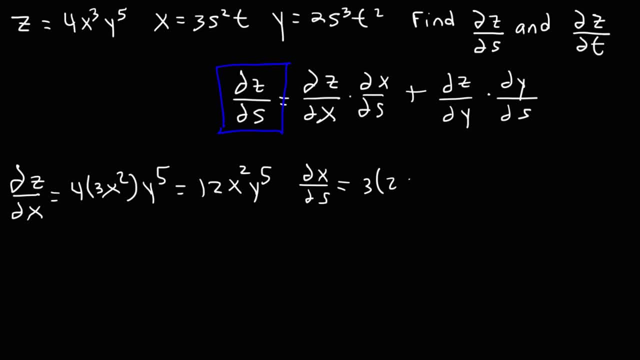 So all we need to do is take the derivative of s squared, which is 2s, And so this is going to be 6st. Now let's calculate the partial derivative of z with respect to y. So x cubed will be treated as a constant. 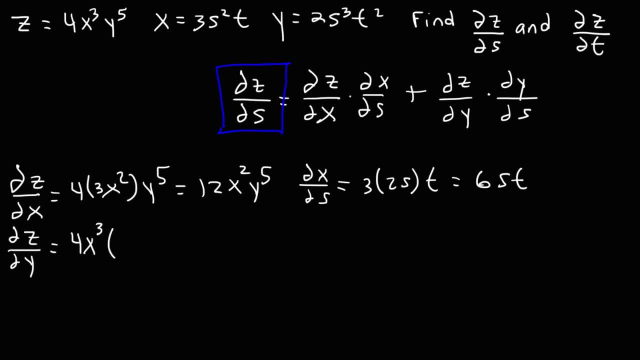 So it's going to be 4x cubed times the derivative of y to the 5th, And that's 5y to the 4th power. So 4 times 5 is 20, giving us 20x cubed y to the 4th. 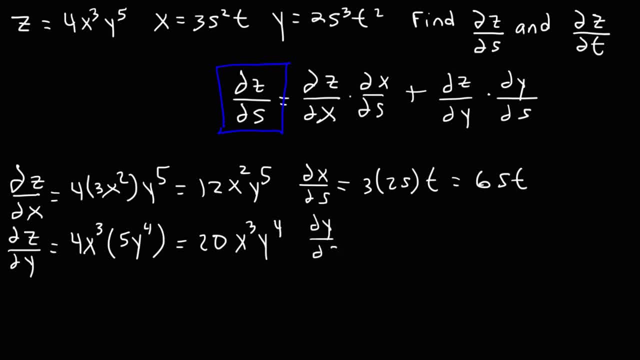 So now we need to find the partial derivative of y with respect to s. using this, So t squared will be 4x cubed, y to the 4th And that's going to be held constant. So it's 2 times the derivative of s cubed, which is 3s squared. 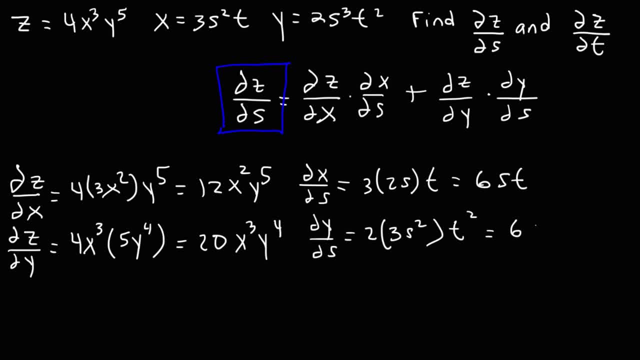 times t squared. So that's 6s squared t squared. So now let's plug in everything into this formula. So the partial derivative of z with respect to s is going to be this part, which is equal to 12x squared y to the 5th. 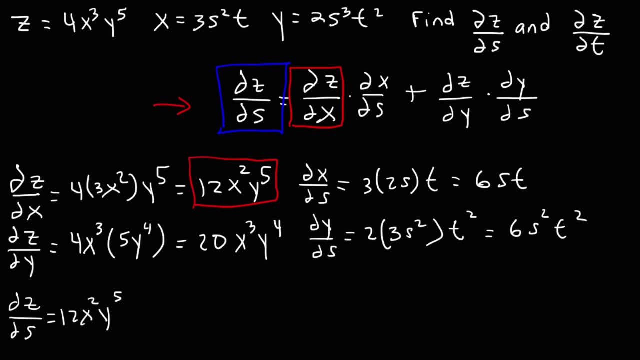 And then that's going to be multiplied by the partial derivative of x with respect to s, So that's 6st, And then plus, So we have this right here. That's equal to 20x cubed y to the 4th. 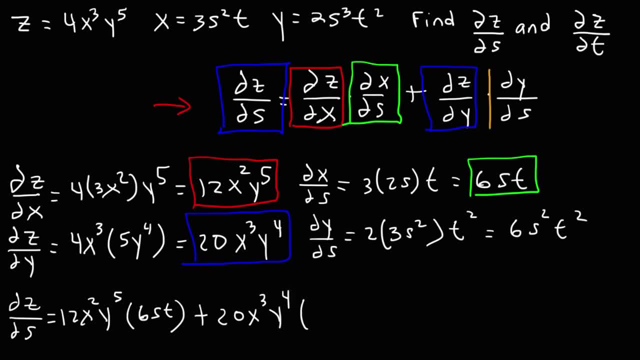 And finally, the partial derivative of y with respect to s, which is 6s squared t squared. So our answer is going to be 12 times 6,, which is 72.. x squared- y to the 5th power st. 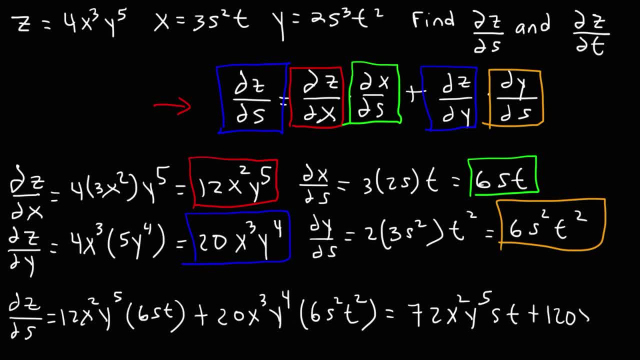 And then 20 times 6 is 120.. And then x cubed y to the 4th, s squared, t squared. So this is our answer: The partial derivative of z with respect to s. Now, if you want to, you could replace x with 3s squared t. 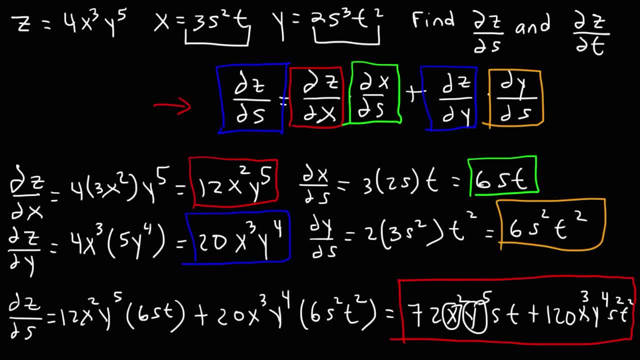 And you could replace y with 2s cubed t, squared, So you can get the partial derivative of z with respect to s in terms of s and t. if you want to eliminate x and y, All right, But I'm not going to do that here because, as you can see, 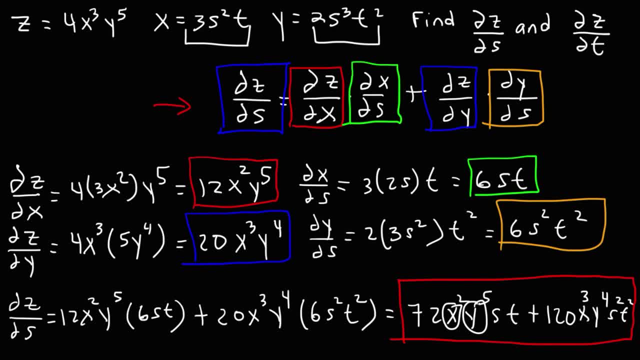 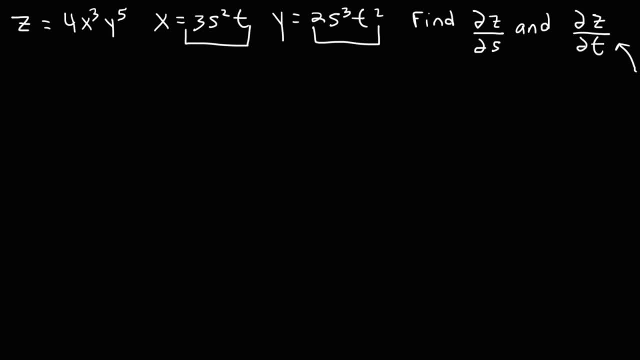 I am running out of space. Now let's do the other part of this problem. So let's find the partial derivative of z with respect to t, And you could pause the video and try that problem yourself. So let's begin with the tree diagram. 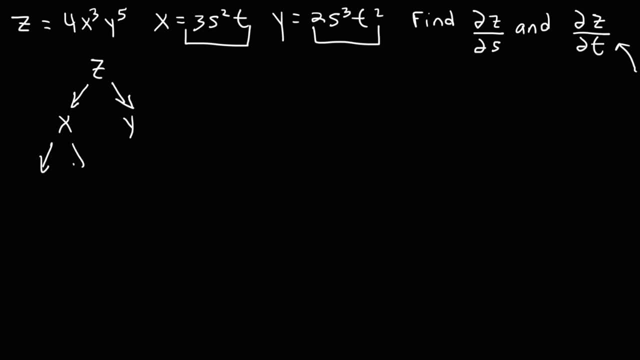 So z is a function of x and y. x is a function of s and t, And the same is true for y, One space. We also find the area ofчивaires to be a abe, a common denominator of z and x squared t. So x squared t, Three points of z squared t, And here we even have it. So we have thedon't actually get this straight, And we have t squared squared t, And we have t squared squared t, So one space. So our focus is now on the t variable as opposed to the s variable. 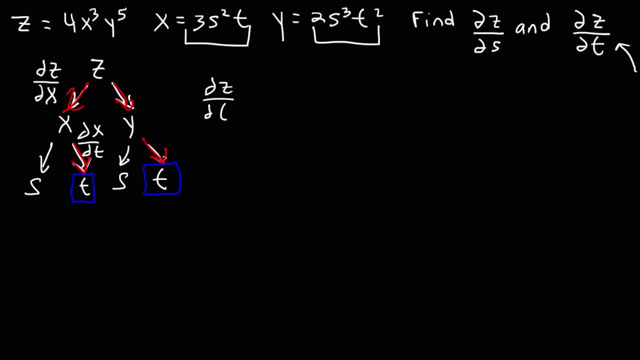 that the partial derivative of Z with respect to T is going to be the partial derivative of Z with respect to X times the partial derivative of X with respect to T, and then plus next is going to be the partial derivative of Z with respect to Y, and then the partial derivative of Y with respect to T. 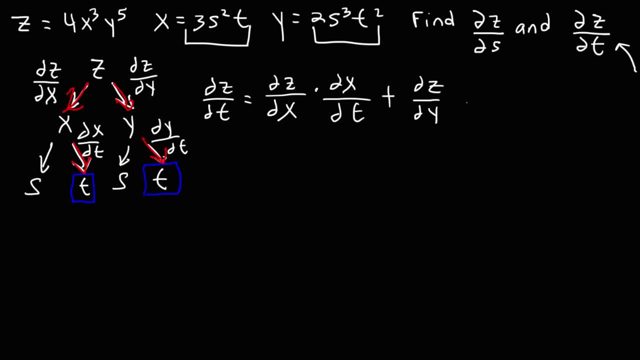 and so that's going to be it. so now let's do the math. let's start with the partial derivative of Z with respect to X. so we did this already. it's going to be 4 times 3x, squared Y to the fifth, so that's 12x squared Y to the fifth, and the partial derivative of Z with. 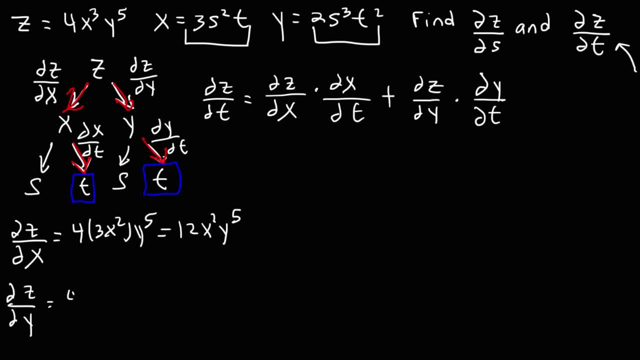 respect to Y, it's going to be 4x cubed times 5y to the fourth, and so that's 20x cubed Y to the fourth. now this is going to be new: the partial derivative of Z. I mean of X rather to T. so we're using this and S squared will be treated as a constant. so it's. 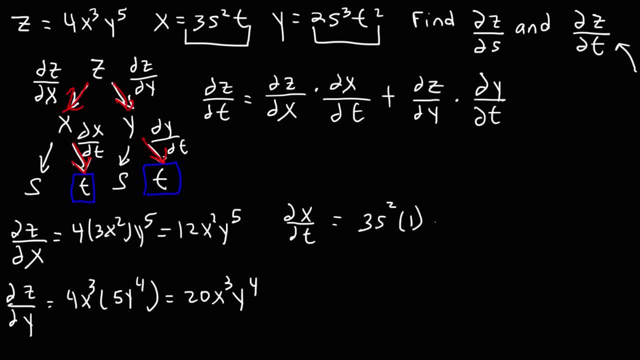 going to be 3s squared times the derivative of T, which is 1, so that's just 3s squared and the partial derivative of Y with respect to T. it's going to be 2s cubed. and then times the derivative of T squared, which is 2t, and 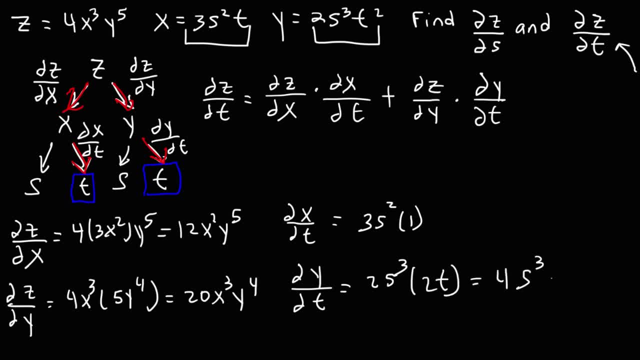 so that's going to be s cubed t. Now let's put this all together. So the partial derivative of z with respect to t is going to be the partial derivative of z with respect to x. So that's 12 x squared y to the. 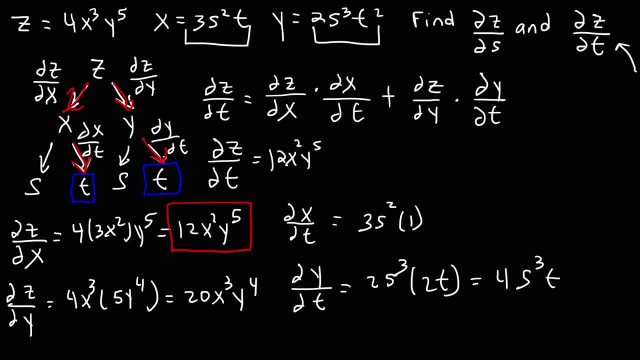 fifth, power, and then times the partial derivative of x with respect to t, So that's times 3s squared, and then plus the partial derivative of z with respect to y, So that's 20 x cubed y to the fourth, and then the last one, the partial derivative of y with 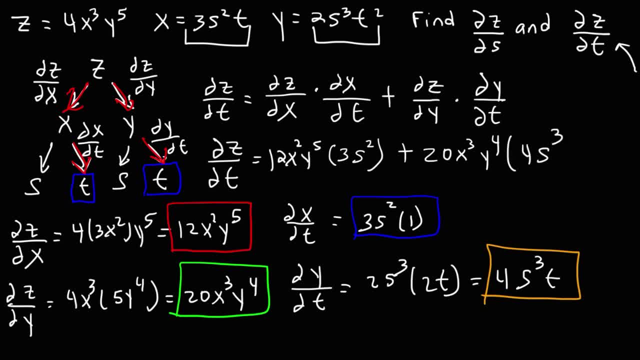 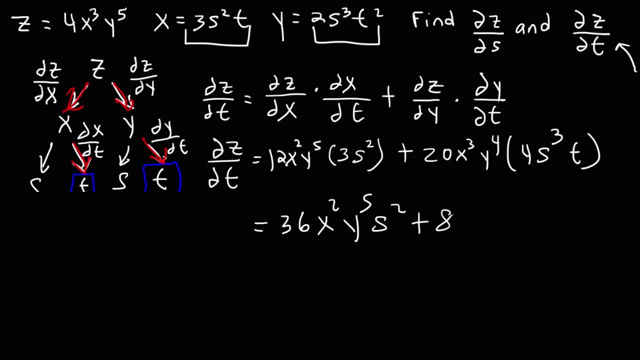 respect to t, That's going to be 4s cubed t, So the final answer is going to be 36 x squared t y to the fifth times s squared, plus 80 x cubed y to the fourth s cubed t. 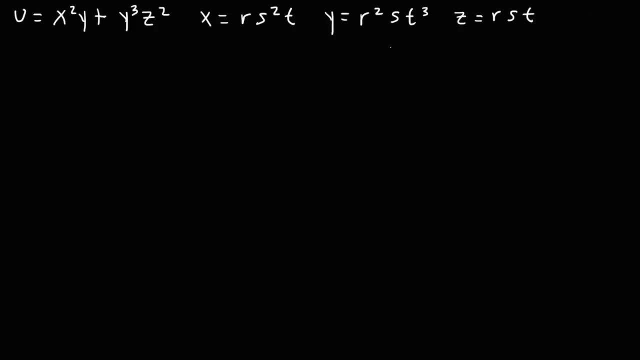 So that is the answer for this problem. For the sake of practice, let's work on one more example. So we're given the function of u, x, y and z and we want to find the partial derivative of u with respect to t. Go ahead and try that. So let's begin with a tree diagram. So u is dependent on three variables: x. 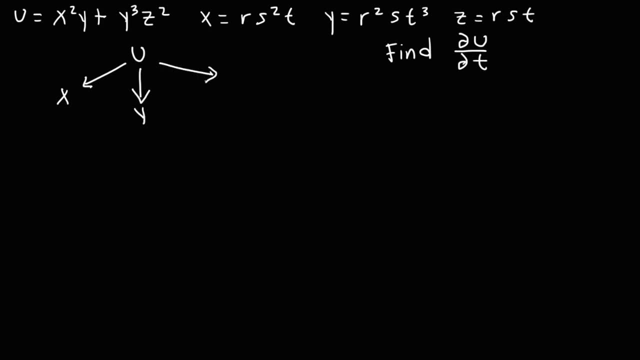 y and z. Now, x also depends on three variables. It depends on r, s and t. The same is true for y and the same is true for z. Now, since we're looking for the partial derivative of u with respect to t, we're going to focus on the t variables. 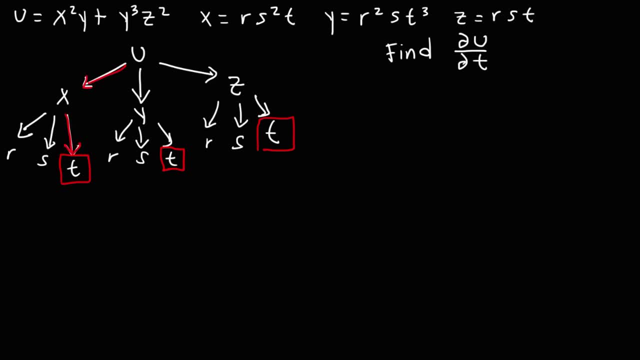 So let's start with this path and let's write the formula. So the partial derivative of u with respect to t is going to be the partial derivative of z. So let's start with this path and let's write the formula: The partial derivative of u with respect to x. 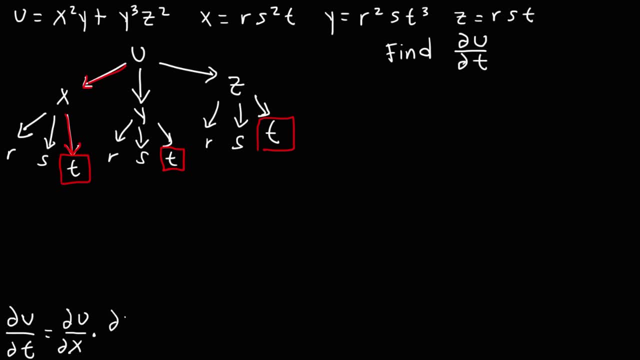 times the partial derivative of x with respect to t. Now, let's take this path. So we're going to have the partial derivative of u with respect to y times the partial derivative of y with respect to t And finally, for the last one, this is going to be the partial derivative of u with respect to z times the partial derivative. 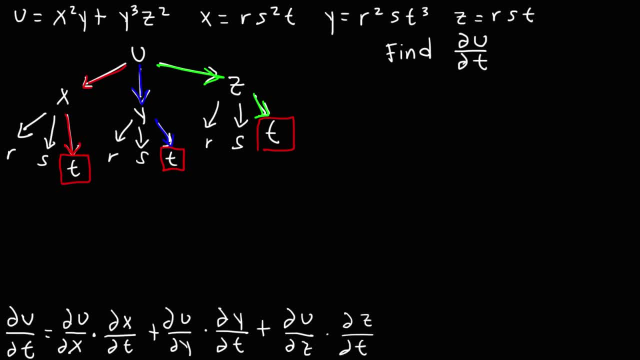 of z with respect to t. So that's the formula that we need to use. Now let's get everything that we need. So let's begin by finding the partial derivative of u with respect to x. So y and z are going to be constant. The derivative of x squared is 2x times y And 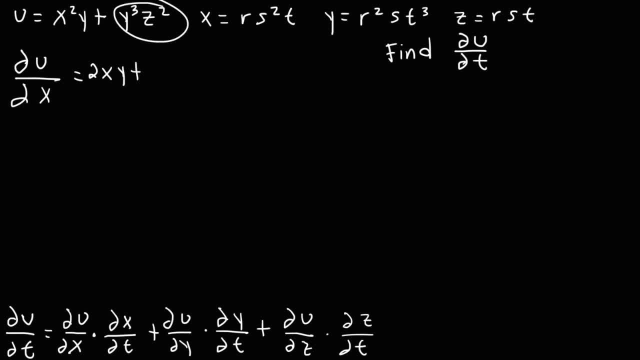 notice that there's no x variables here, So that whole thing is a constant. The derivative of a constant is 0.. Now let's find a partial derivative of x with respect to t. So that's using this formula. So r and s, squared are constants. The derivative of t is 1, so we just get rs squared Now. 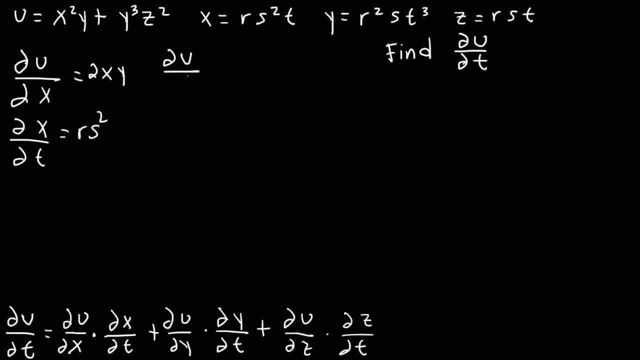 let's find the derivative of the partial derivative of u with respect to y. So, using this equation again, it's going to be the constant x squared times the derivative of y, which is 1,, plus the derivative of y cubed, which is 3y squared, and then times z squared. 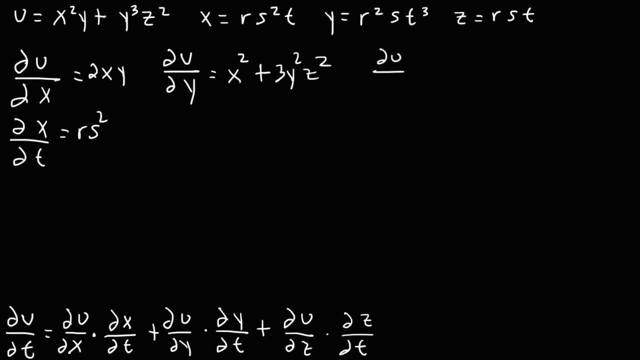 Now let's go ahead and find the partial derivative of u with respect to z. So this doesn't have a z variable. that's going to be 0.. And then it's going to be y cubed times the derivative of z squared, which is 2z, And so this is 2 times z times y cubed. Now let's find the. 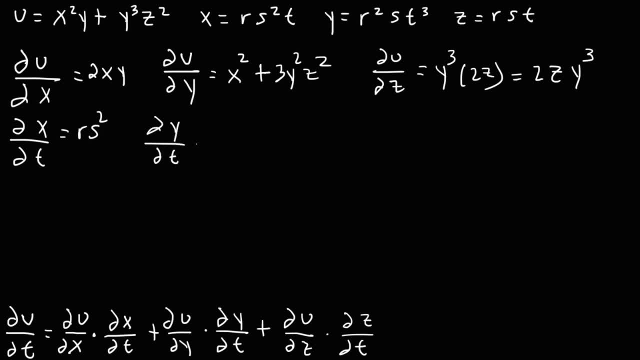 partial derivative of y with respect to t. So using this formula, we're going to get the partial derivative of u squared times the derivative of z squared, which is 2z. So let's find the partial derivative of y. Now let's look at this equation one by one. Let's see: 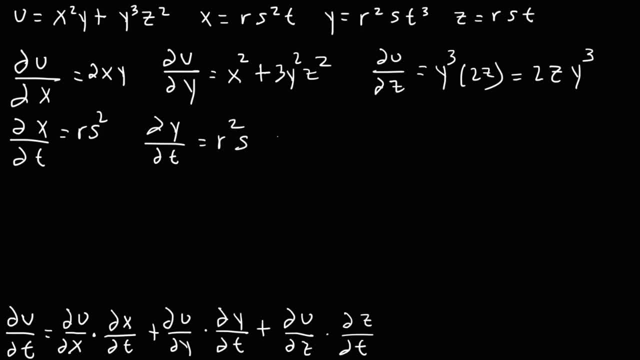 the r squared s part will stay the same. the derivative of t to the third is 3t squared. now the partial derivative of z with respect to t is going to be rs times the derivative of t, which is 1. so at this point we have everything that we need.